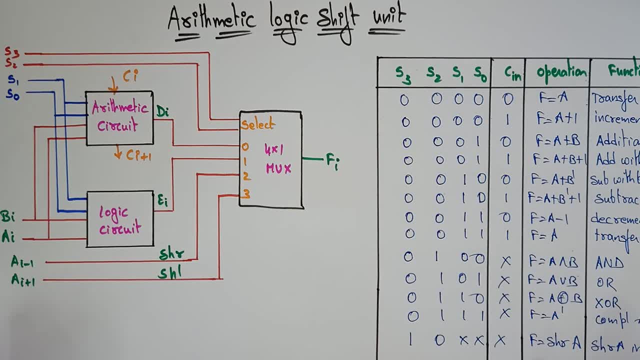 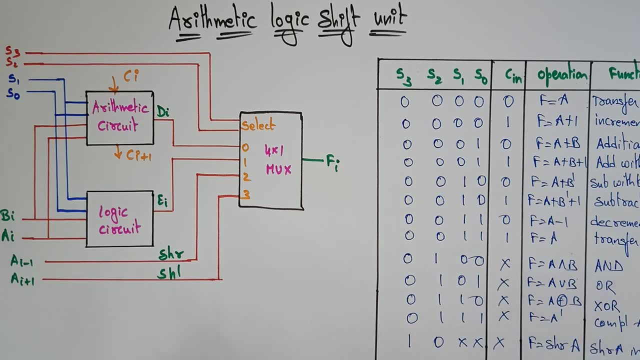 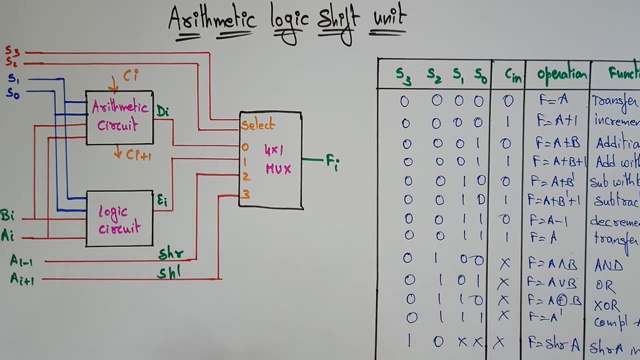 Hi students, welcome back. Coming to the next topic in the subject, computer organization and architecture, is arithmetic logic shift unit. So here I had drawn the digital circuit and the operations that this circuit is going to be performed. Okay, let's start. So if you see this, 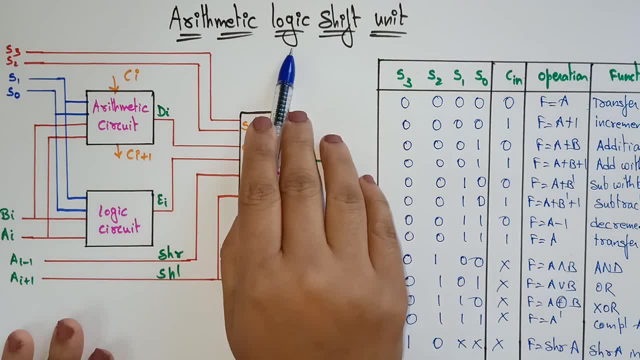 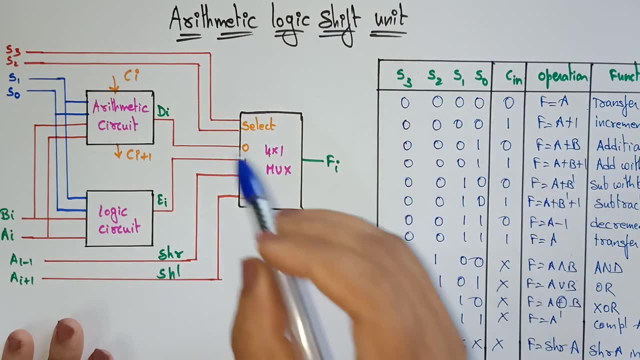 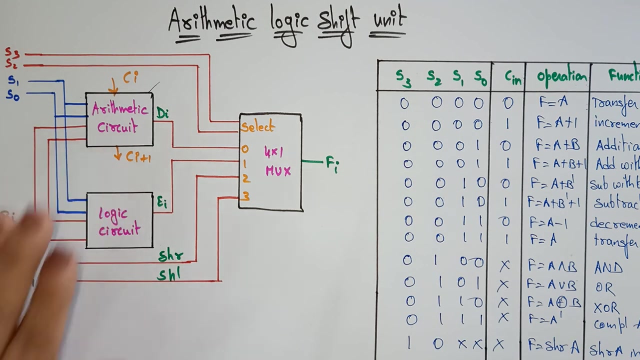 here. this is a circuit of arithmetic logic shift unit. So here we are performing, that is, this digital circuit that performs arithmetic calculations. it is performing arithmetic calculations, logical manipulations as well as shift operations, So all three it is going to be performed. So this circuit- again I am repeating students- this arithmetic logic shift, the name: 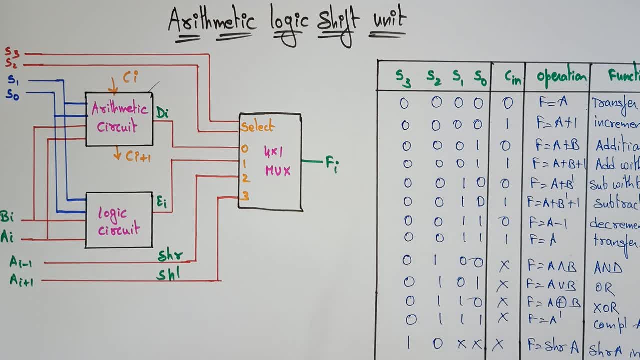 itself it is saying that it is going to perform three kinds of operations Rather than single operation. this circuit is providing three types of operations. It is doing arithmetic calculations, logical manipulations and the shift operations. Okay, so, if you see this diagram carefully, this block diagram of arithmetic logic unit includes: 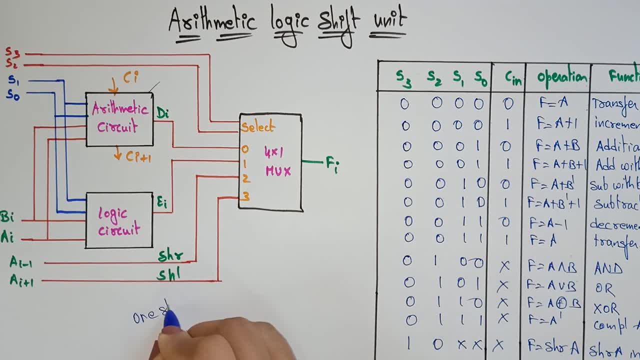 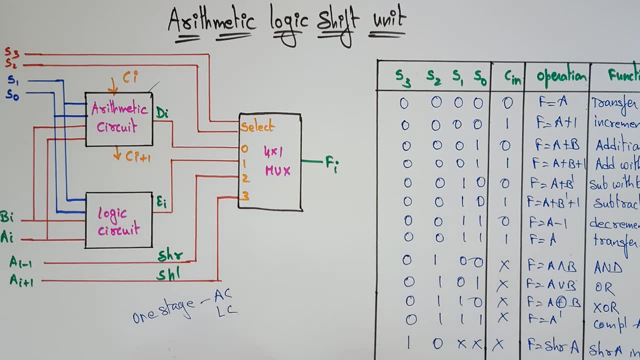 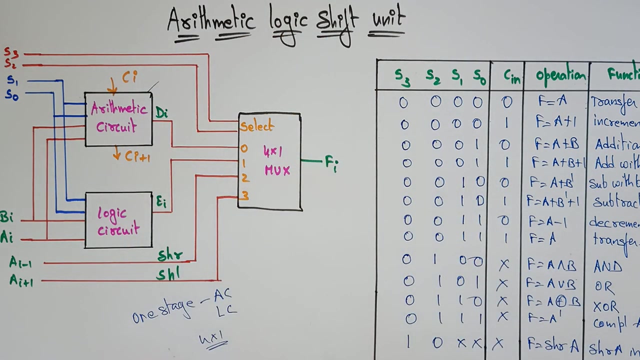 only one stage. We call it as a one stage of arithmetic circuit, logic circuit as well as, and shift manipulations, shift instructions and one four by one multiplicator. so it is having one four by one multiplexer and only one stage of arithmetic circuit and one stage of logical circuit. What does it mean? 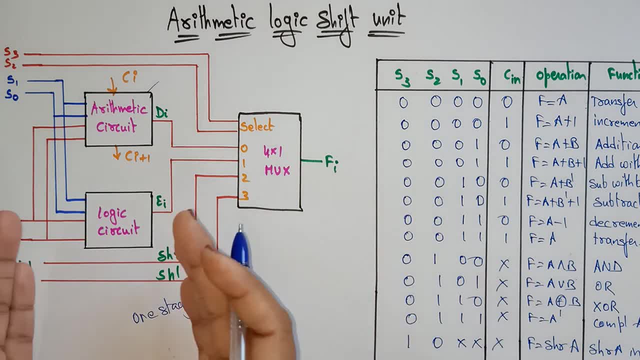 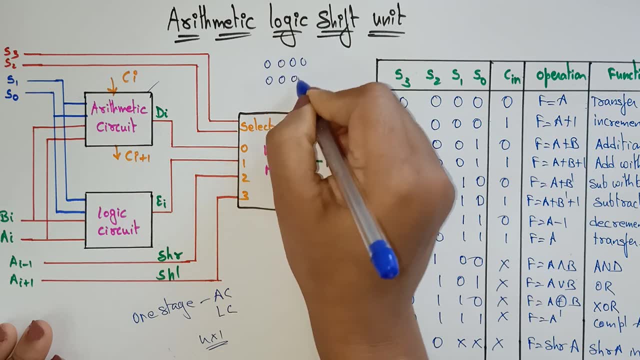 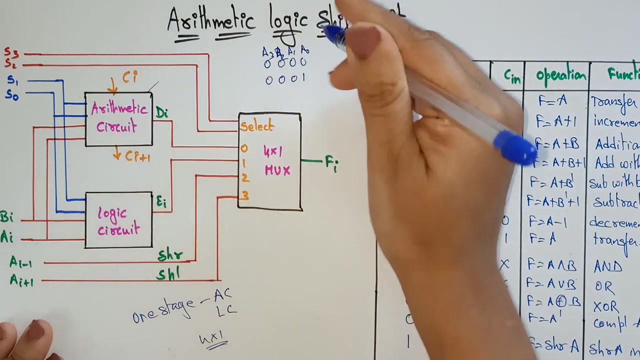 only one stage you're able to see here. Suppose if you're having four bit like 0, 000.. Something like this is a 4 bit. so this is a, not a1, B1, sorry, A2A1, A2.. A3.. So this is the each bit. So here we are showing the circuit, only with A0, only with A0.. 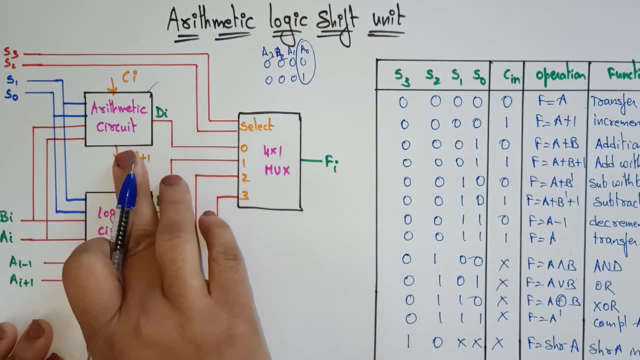 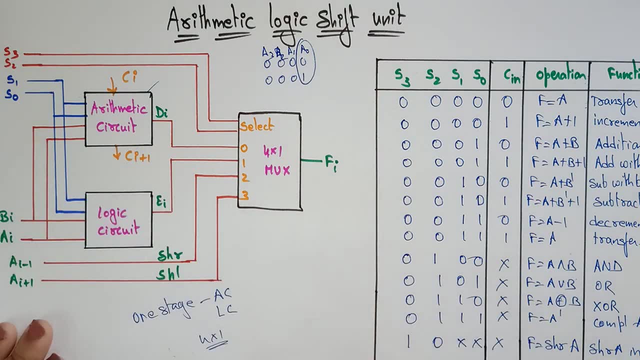 So that is one stage and this will be connected with another stage means that is A1 and again, if you are connecting with that is a two stage and three stage and four stage, like that you can see. but in this diagram we are only showing the one stage: arithmetic logic shift unit. Now let's have 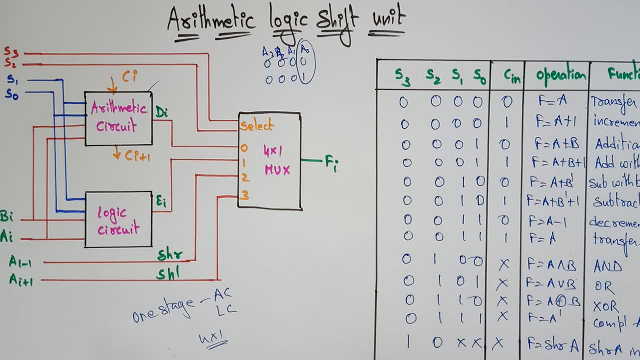 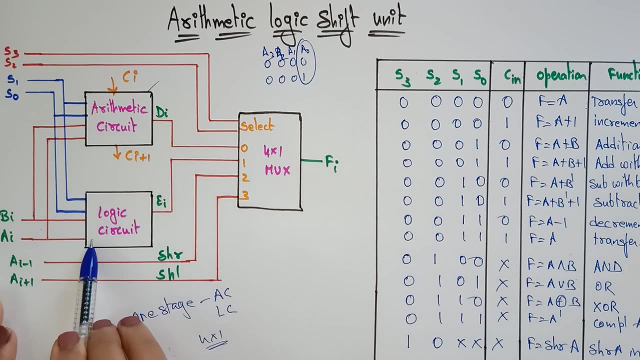 a look on what exactly this arithmetic logic shift it is going to do Coming to here. these are AI and BI. these are the inputs. So these are inputs to given to arithmetic circuit. if you clearly observe, this input is given to arithmetic circuit as well as a logical circuit, not for the shift. 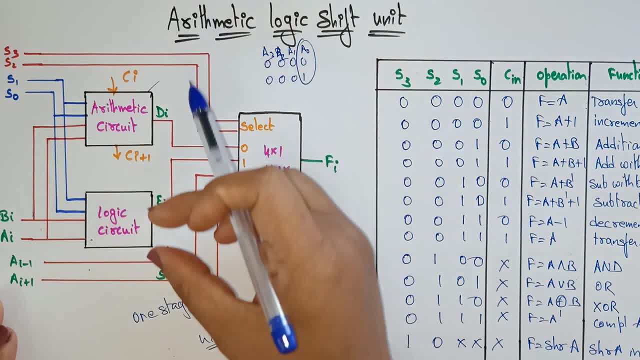 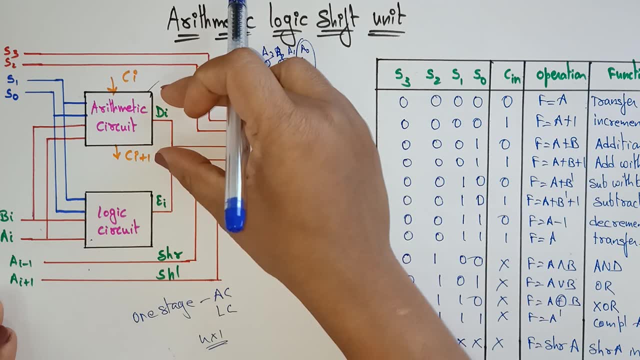 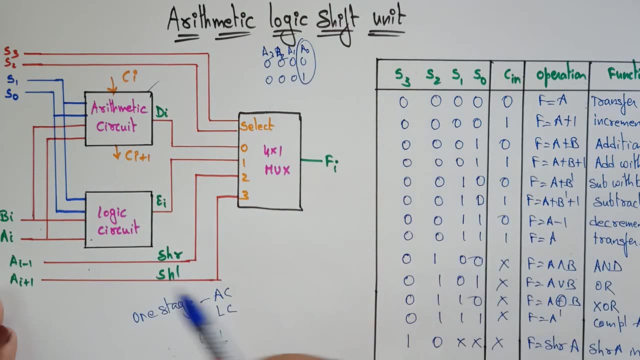 So AI BI can be perform either in arithmetic or in logical circuit. One thing, students, you have to remember: at a time only one unit can be activate. Both units cannot. both circuits cannot do the operations at the same time. So whenever the values that we are given, either these AI BI will be work for. 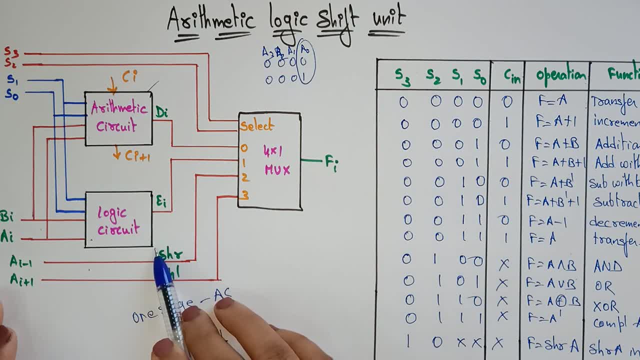 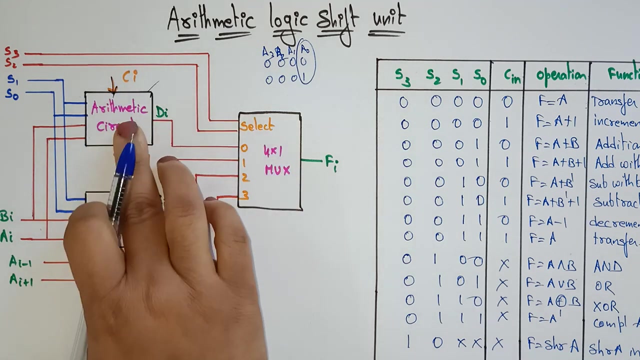 arithmetic circuit or it can be logical circuit. So both operations cannot perform at a time either. arithmetic, Any one can perform at a time by using this two input: A, I and B I. and here, if you see, this is the carry bit. The carry bit is connected to the. it's an input to the arithmetic circuit, AI, BI and the CI. So three inputs are. 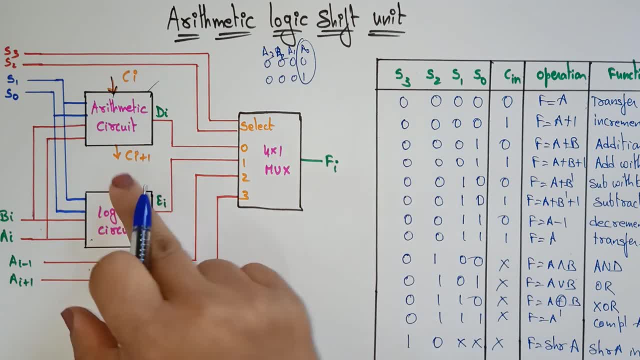 giving to the arithmetic circuit and another carry. If suppose, if you perform A plus B plus C, A plus B is the input and C is the carry. if again, if you get the carry, that carry will be connected to the next stage of the arithmetic logic unit. 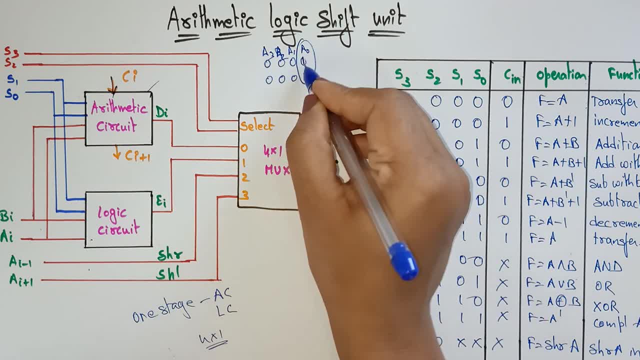 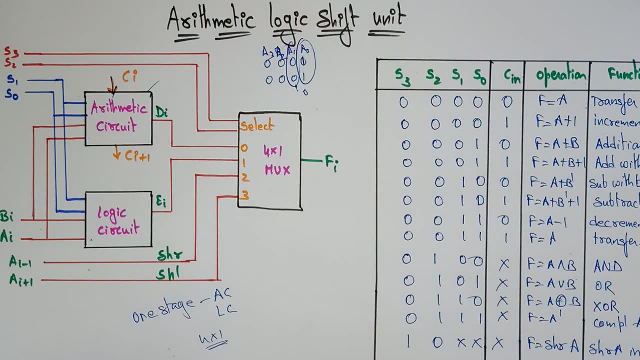 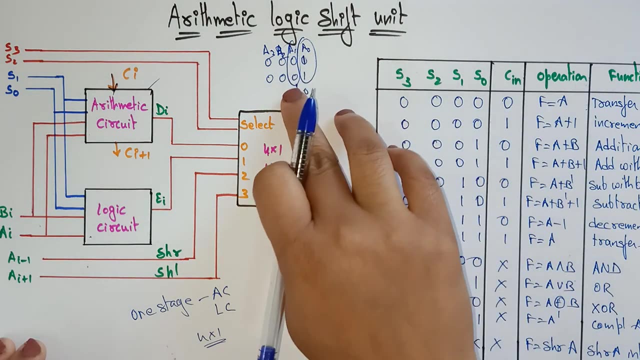 okay, that means here, if you perform, suppose 1, 1 is there, okay, carry is get. so this will be connected to the next stage, the next stage of the l? l. you see, that is arithmetic logic shift unit. and if suppose here, if carry is there, that is ci plus 2, that will be connected to the next stage. 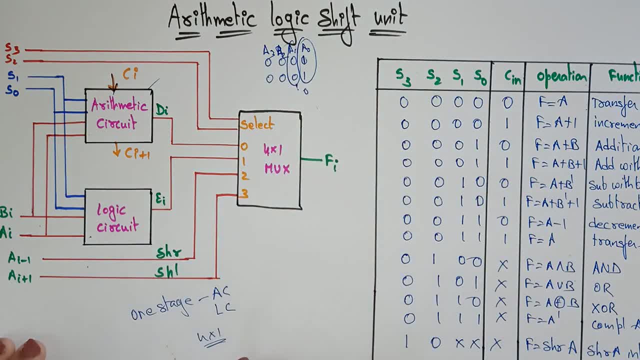 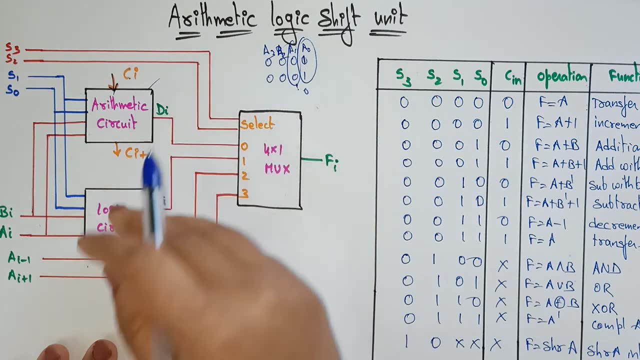 and ci plus 3, that will carry will be connected to the next stage. so that is what here it is happening. so diagram a: carry will be connected to the arithmetic circuit, but for the logical circuit there is no carry. the carry bit is provided to one stage of au. that is the sorry. 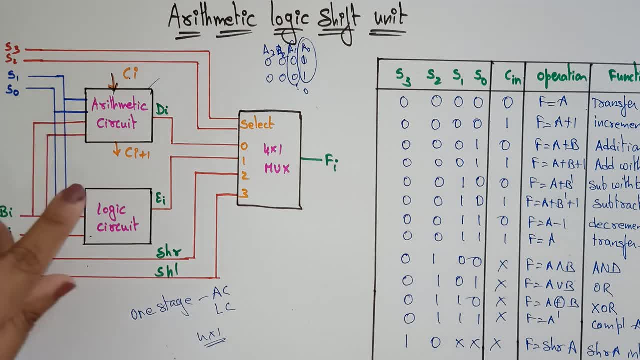 arithmetic circuit ci and the corresponding will be get ci plus 1, and logic circuit does not require any carry operation. this point you have to do the same thing. you have to do the same thing. you have to do the same thing. you have to be remember that only arithmetic circuit is having the, is holding the carry, but logic 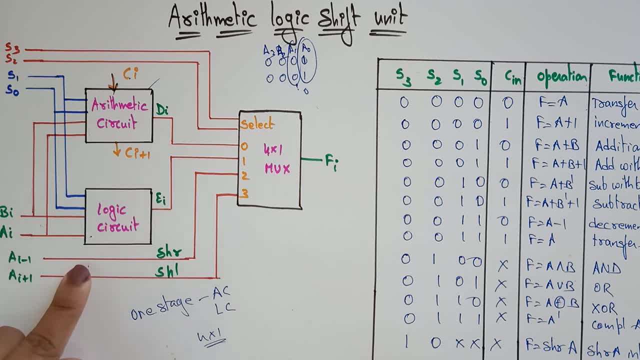 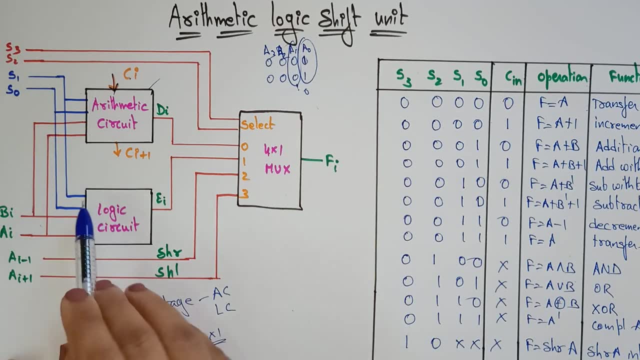 circuit will does not require any carry operations. and if you see here these are the four select lines, are there s1 and s2? s? naught is provided for both units. so these two bits are identifying s? naught and s1. so which input i need to be take either ai or b? i. so what we have to take, 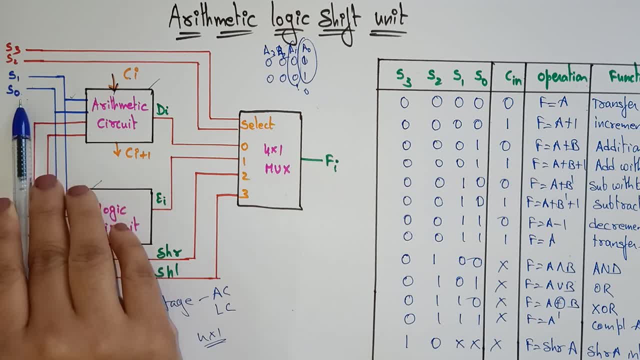 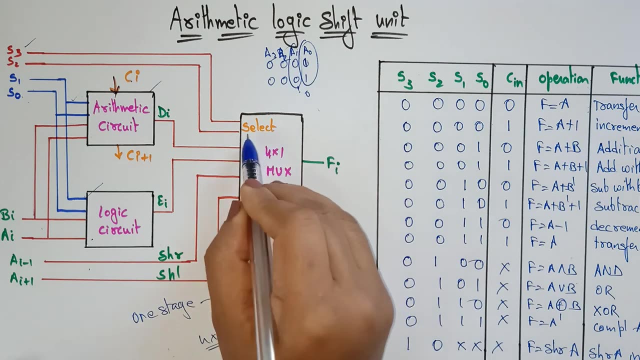 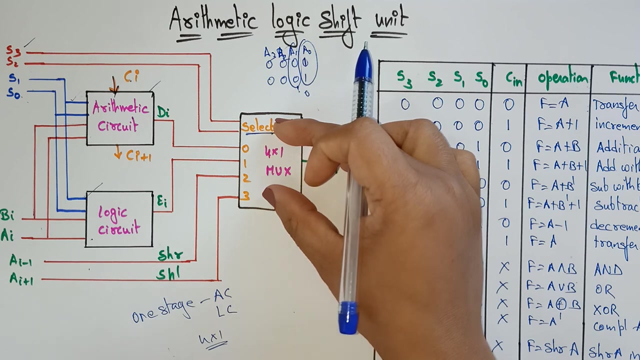 so this is the selection bits s1 and s naught. so these two select lines will be provided connected to the arithmetic circuit as well as the logic circuit, and s2 to s3. these are connected to the multiplexer. so here what these will be doing. this is a select operation. the multiplexer is going to select which circuit is in operation. 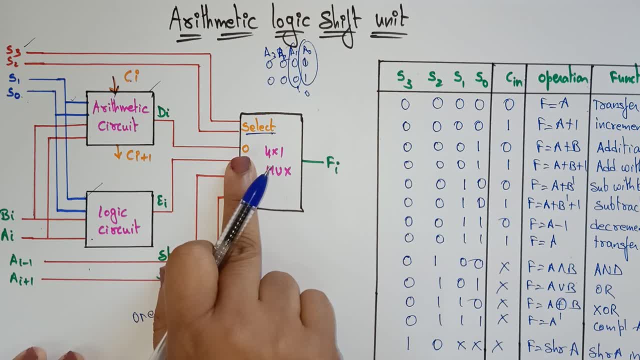 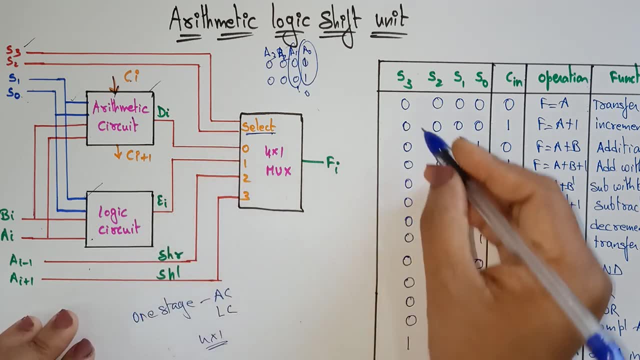 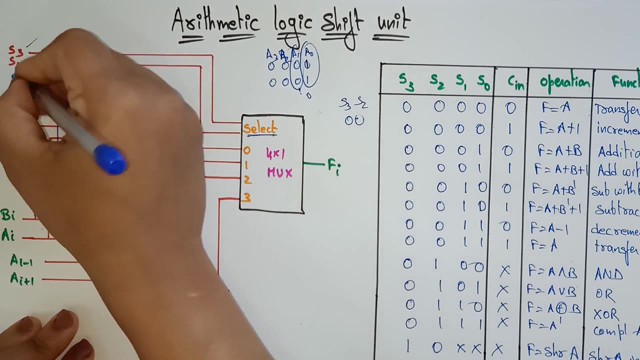 which circuit is providing an input to input to multiplexer, so that can be decided by this select. so suppose the select zero, zero is there if zero, zero is there, that is s3 and s2, both are zeros are there. if these two bits are zero, zero, that means arithmetic circuit is arithmetic circuit is active. 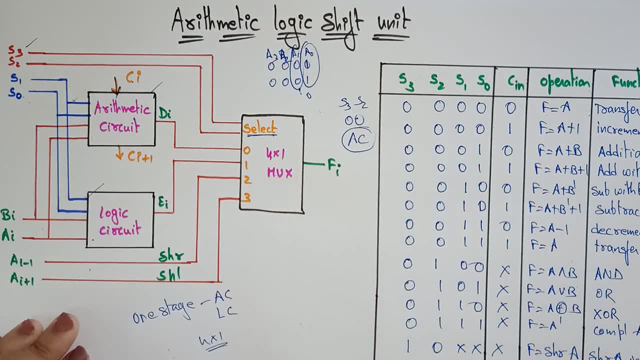 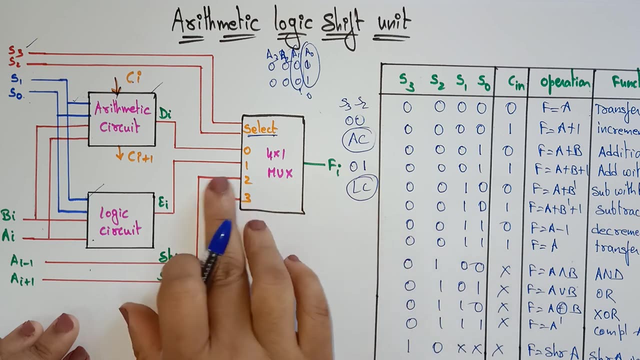 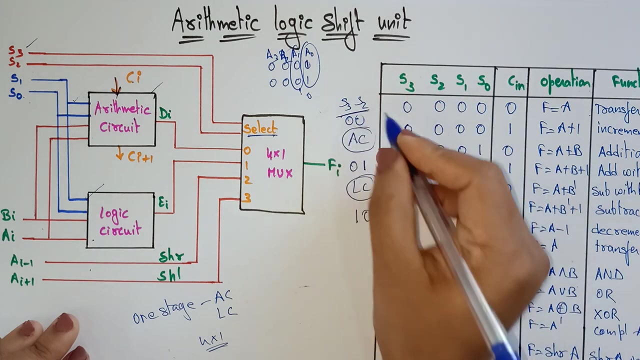 i said, only one circuit will be performing operation at a time. suppose zero one is there- s3 and s2- or zero one is there, that means logical circuit is performing the operation. the input is coming from the logical circuit. suppose one zero is there- s3 and s2, or one and zero. one and zero means a shift right. operation is going to be performed. 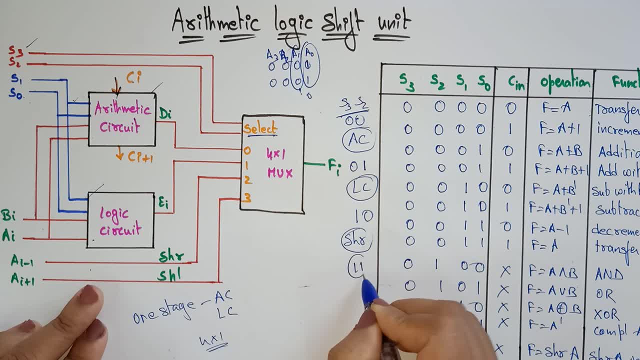 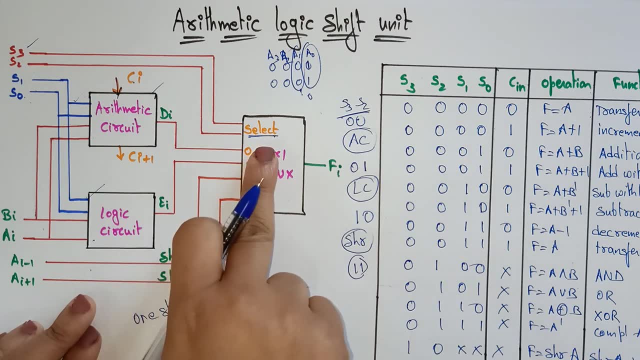 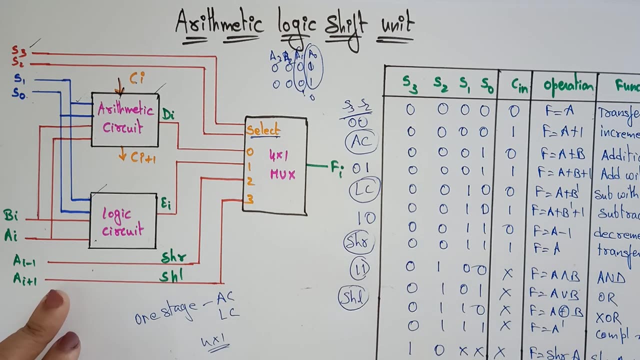 suppose one one is there, one one. so s3 and s2 or one one is there. we are giving it is one one is there. the multiplexer is selected. it is as one one. that means the input is coming from the logical circuit is coming from the shift left, the input is coming from the shift left. so this is how the 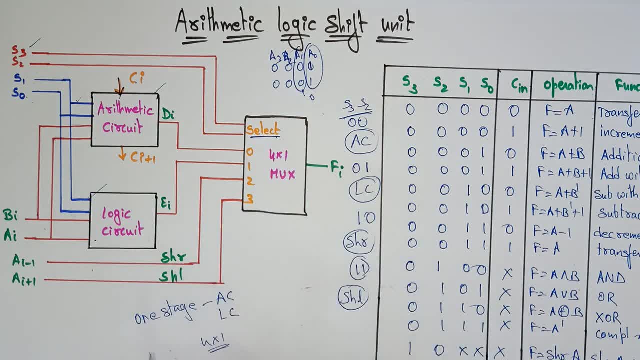 select input is going to be decided which circuit is performing the operation. so one circuit can perform operation at a time. so the input for the shift right is ai minus one and shift left is ai plus one. so we are moving to the left side shifting. so ai plus one you are getting and you 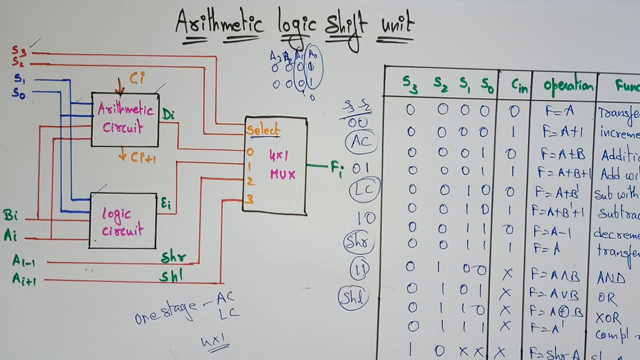 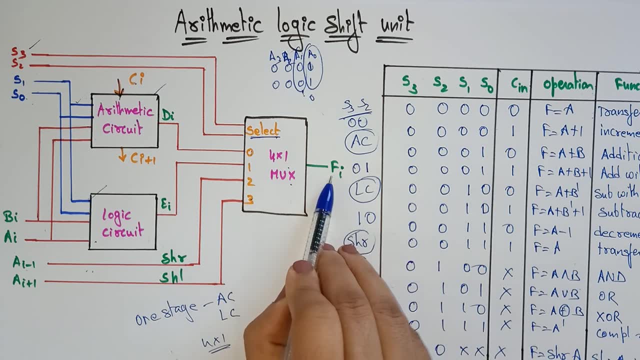 are moving to the right side. ai minus one. it's input. so this is the four by one multiplexer means a four inputs are coming and it is going to generate only one output. that is a function. so what type of operation it is going to perform? either performing the. 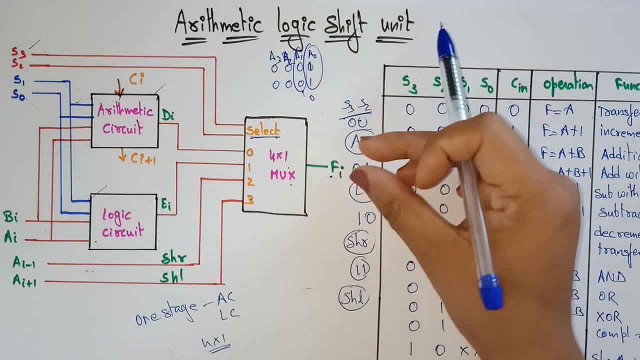 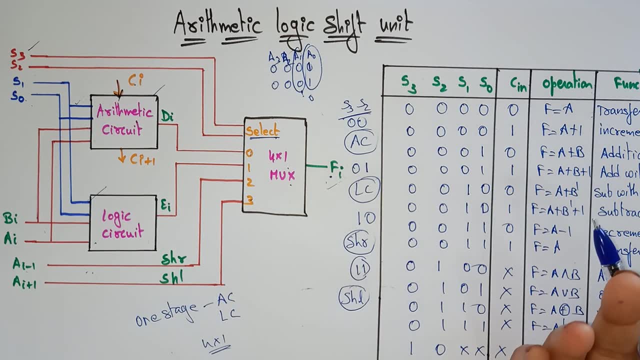 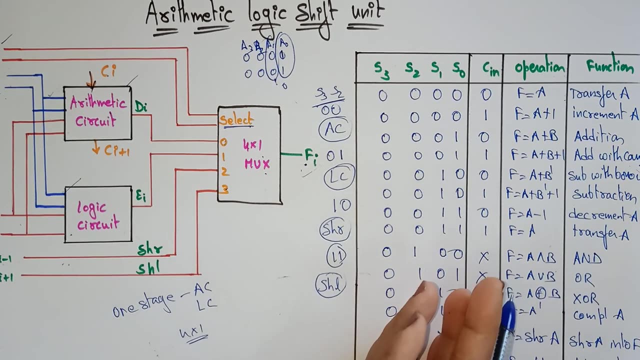 arithmetic operations, or it is performing the logical operations or it performing the shift operations. that will be decided. that will connected to the. that comes from the fi. it's an output. now let's have a look on this table. so we will implement this table in this circuit. okay, so, if you clearly observe, as i said, what i said, uh. 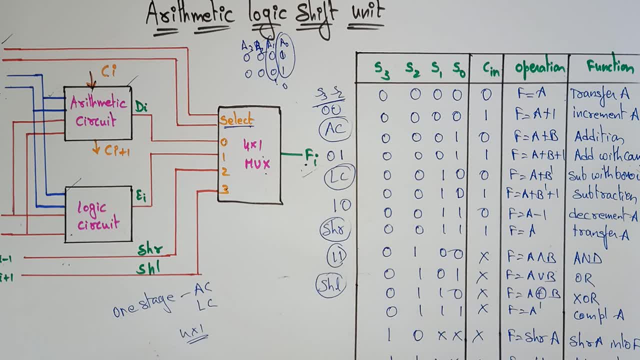 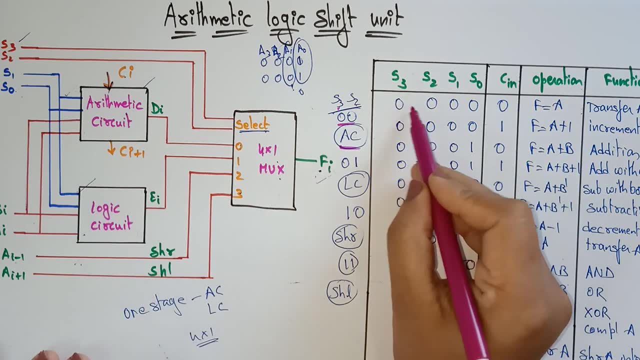 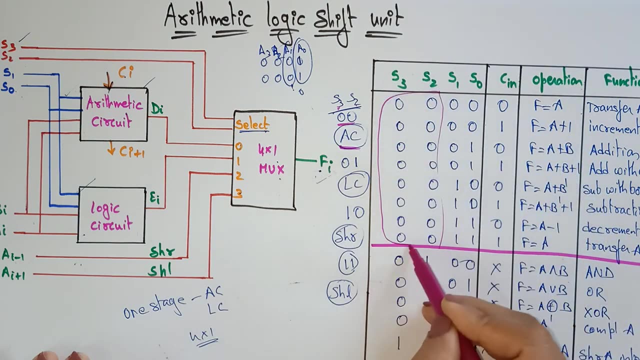 whenever s3 and s2 both are zeros. s3 and s2, both are zeros- only arithmetic circuit is activating. so see here s3, s2 will up. to here: s3 and s2 are all zeros. so whenever these two bits are zeros, that means this: 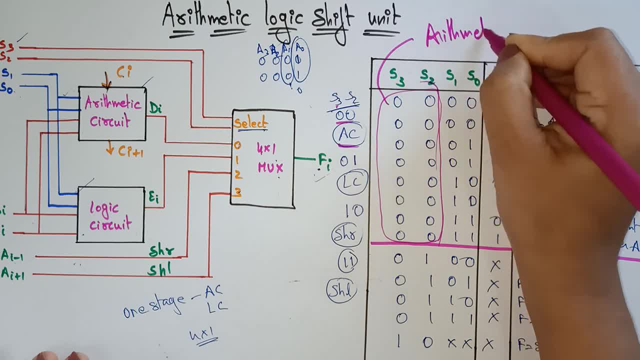 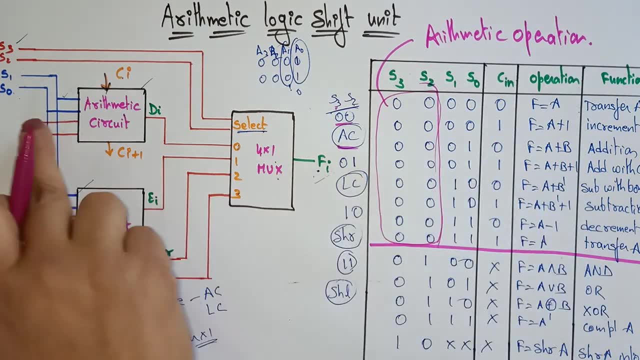 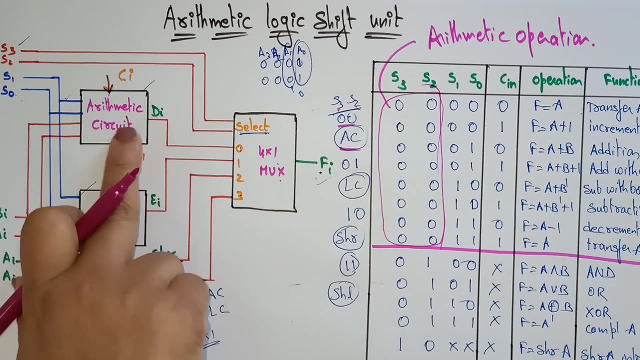 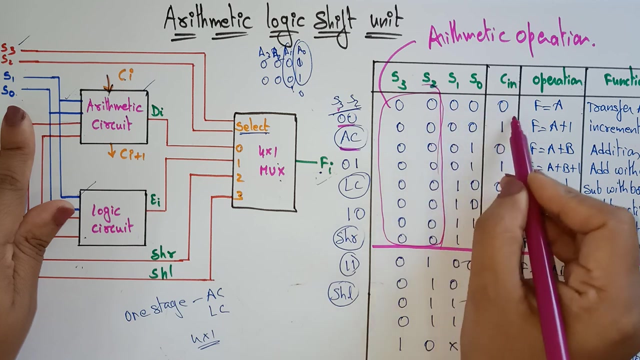 part will be performing only arithmetic operations, so arithmetic operations coming to s1 and s0. so s1 and s0 are connected to the arithmetic circuit. so here logical circuit is not active, only the- excuse me- arithmetic circuit is active. suppose, if you clearly observe, each input will be given twice: zero, zero, zero, zero, zero. 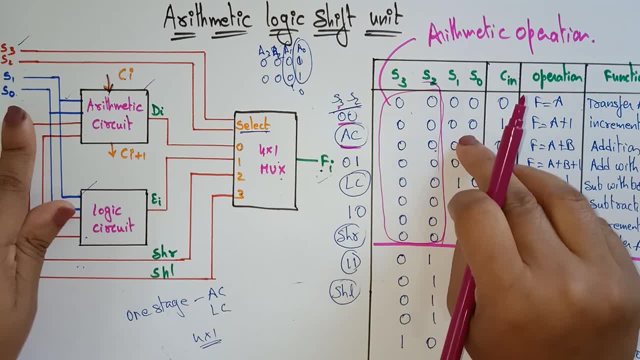 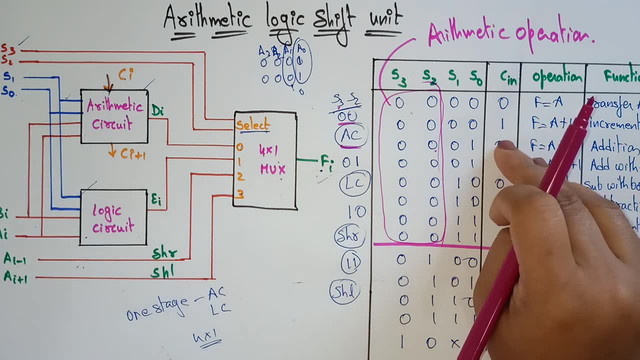 zero, zero, again. zero, zero, one, zero, zero one. why i have given twice? because sometimes the carry may be zero and sometimes carry may be one. it depends upon the uh user uh input that it is given. so if the carry is zero, this operation is going to be. 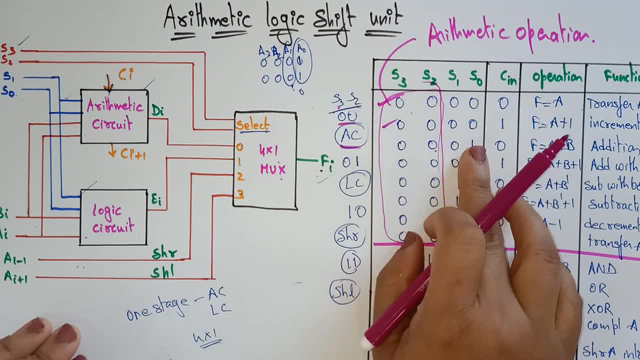 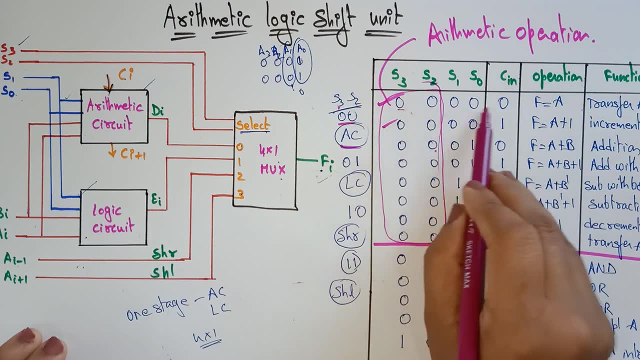 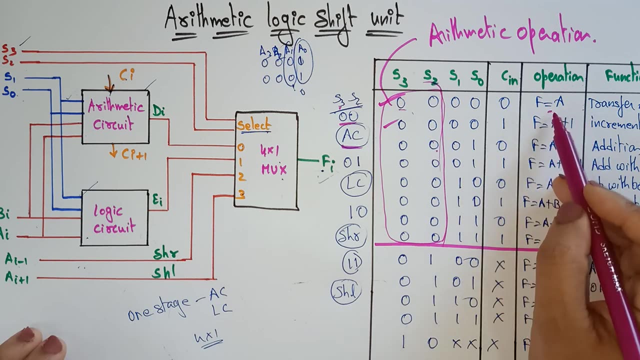 performed. suppose if carry is one, this operation is going to be selected like that: the y, the connection, that is, the bus that is selected based on the carry. suppose if all zeros are there, the operation that you are getting is f is equal to a. that means it's just simply. 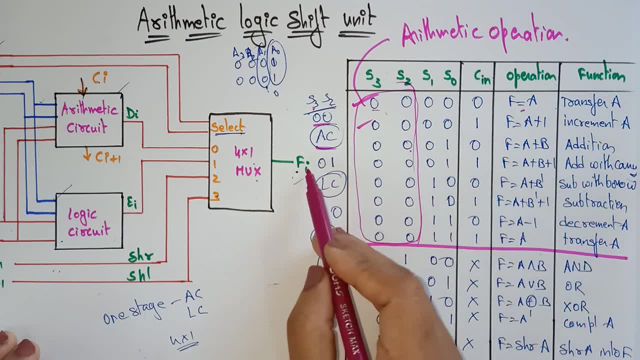 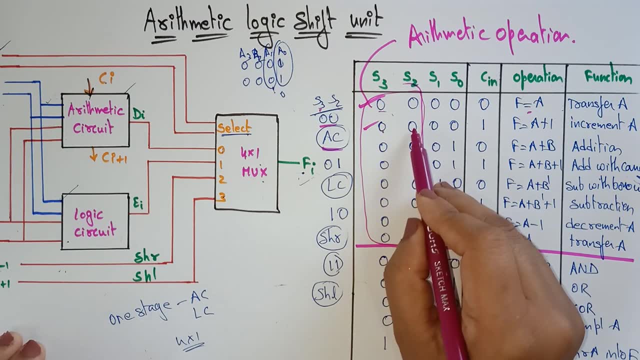 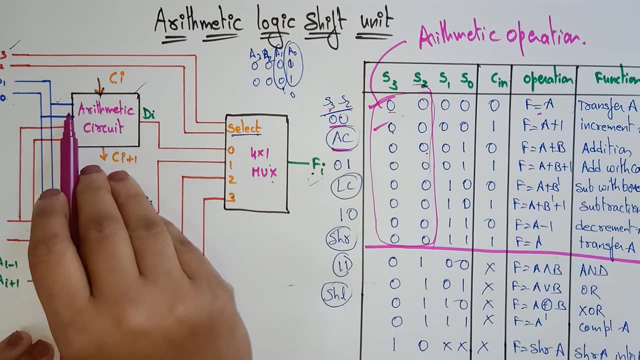 doing the transfer operation, transfer a. so the function that it is performing is transfer a. suppose if s3, s2 is zero, that is arithmetic operation and s1 s naught. both are zeros. both are zeros, but carry here. you are getting one. so here a and b. both are the zeros, a and b. 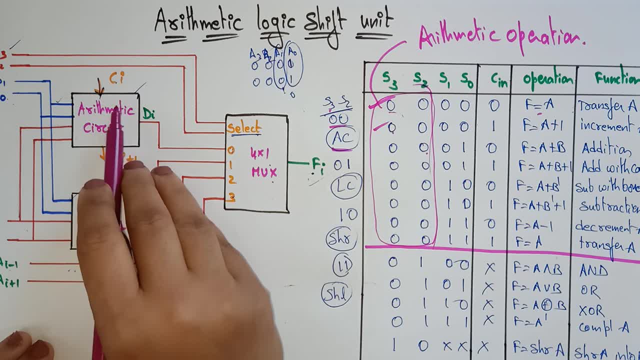 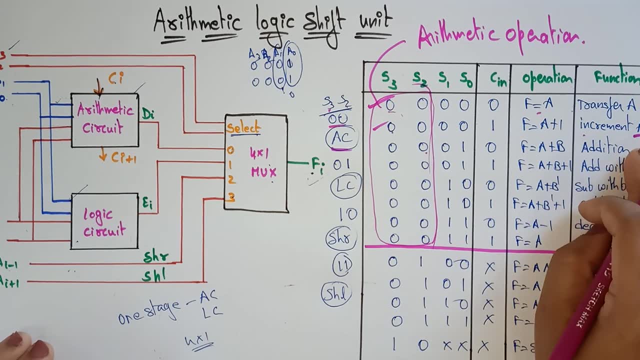 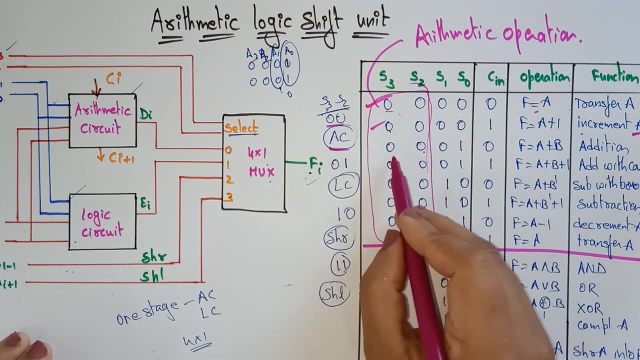 both are the zeros, a naught and b naught. both are the zeros and the carry is one. that means f is equal to a plus one increment a. i'm just adding a to the uh, one to the a, so one to the a. next, if suppose s1 is zero. 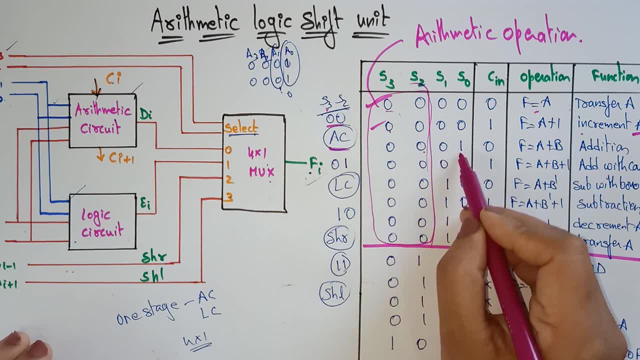 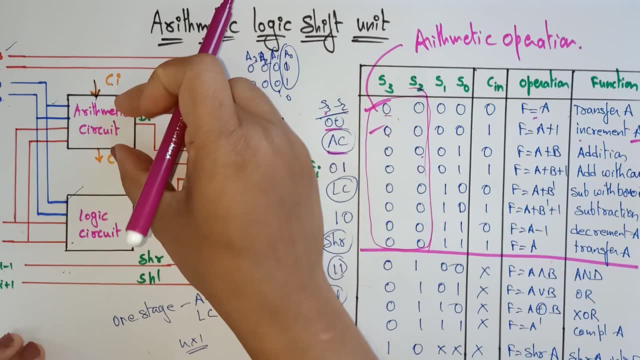 s1 is 0 and s naught is a 1, s naught is a 1 and carry is 0, then it is going to perform addition operation. f is equal to a plus b. only this circuit is performing the operation until s3, s2 are zeros. 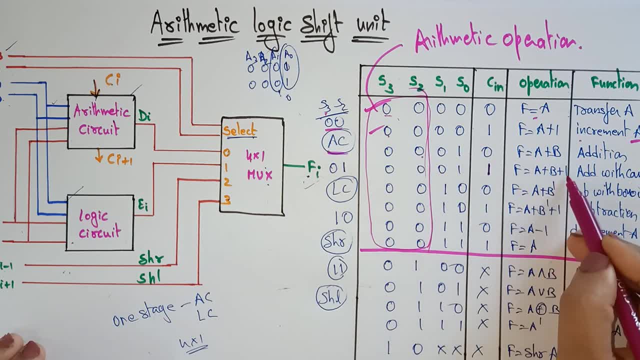 so addition operation. and again, if carry is 1, add, with carry now coming to 1: 0. if carry is 0, f is equal to a plus b, complement operation is performed. and if carry is 1, just add 1. it will do the subtraction operation. 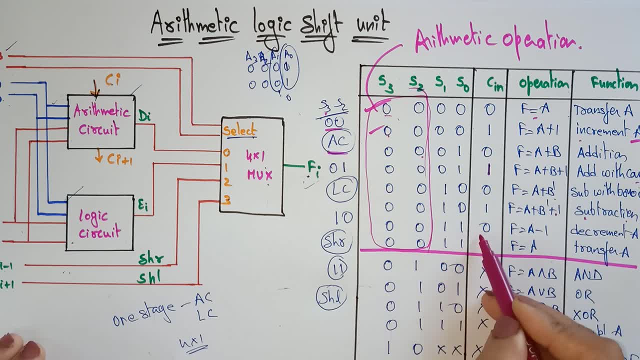 and coming to s1 s naught, both are ones and the carry is 0 means it's just do the decrement operation and if carry is 1 means again transfer a. so this is the operations that is going to be performed by this circuit. according to the operation that is going to be performed by this, 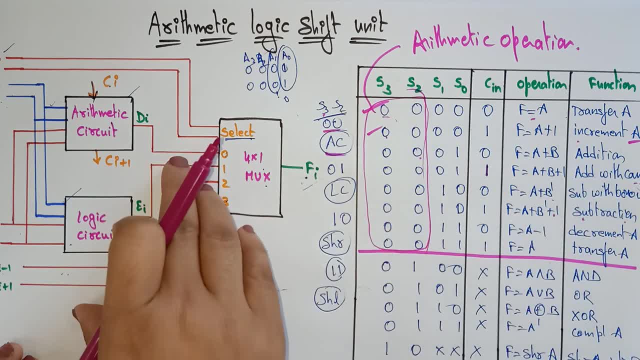 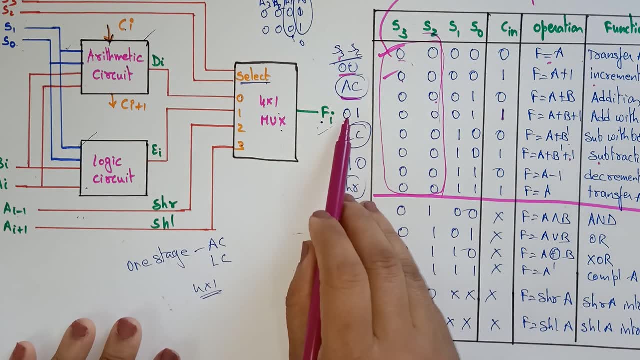 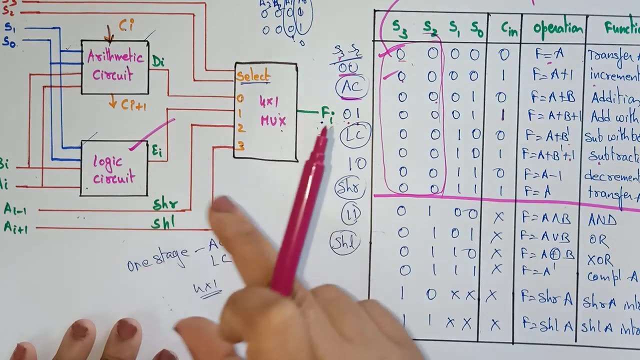 circuit to the. based on the inputs, this circuit is performing the operations. now coming to the logical, what i said: whenever s3 and s2 are 0 and 1, then only the logical circuit is active and the remaining is not performing the operation means they are also. 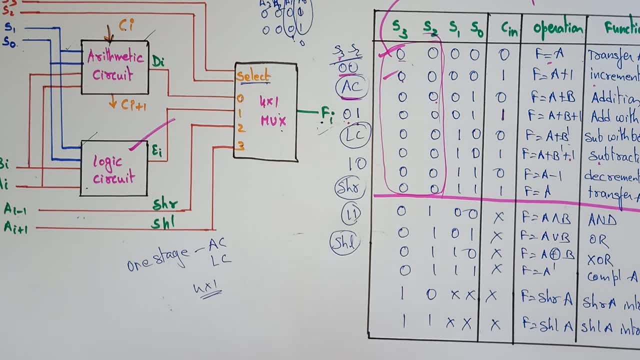 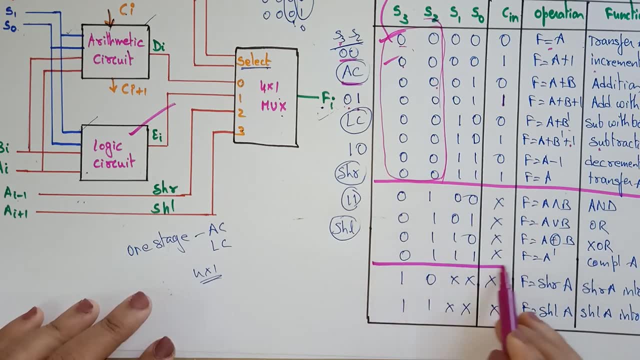 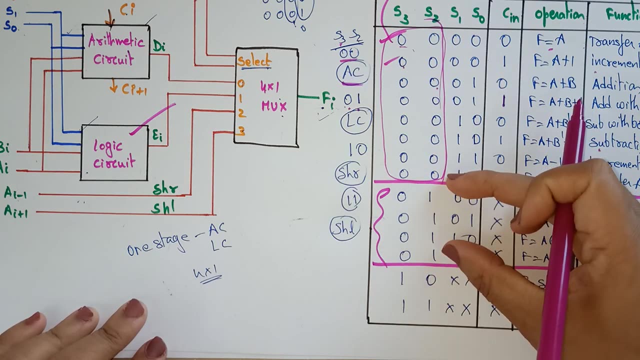 active only, but at a time only one circuit can perform the operation. so the logic circuit is going to perform the operation. so until 0, 1, so this part, 0, 1, this comes. these all four will do the uh logical operations. so what are the logical? 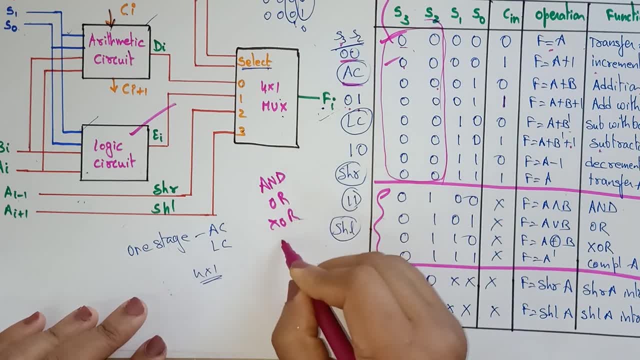 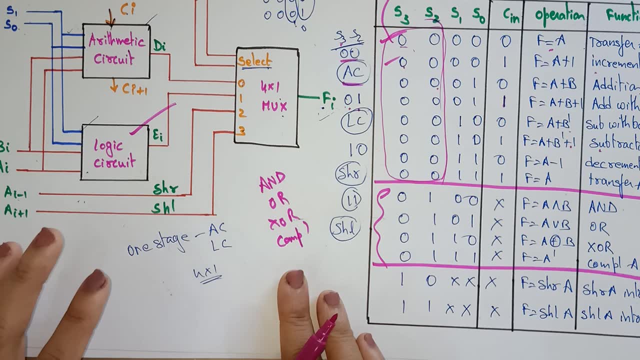 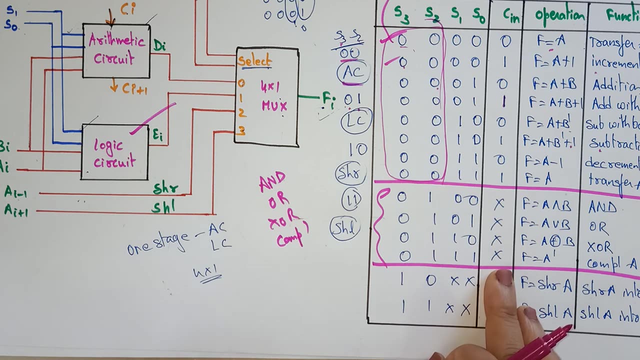 operations and or xor and the complement. so these are the four logical operations. let us take these logical circuit is performing the operation and if you see here the carries don't care conditions because the logical circuit does not require any carry operation. that's why it is everything. it's a don't care condition, okay, so let's go ahead and have a look too at the simple circuit we had said earlier: weAM9aiH8a那我們. 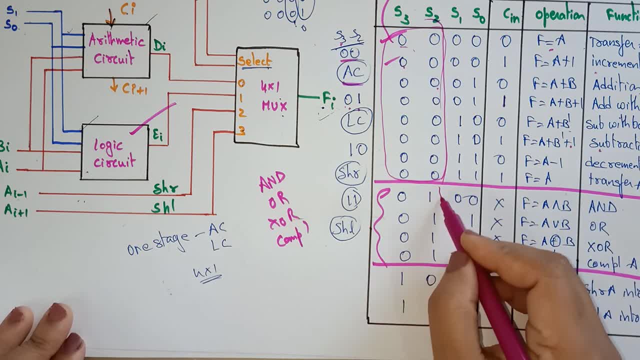 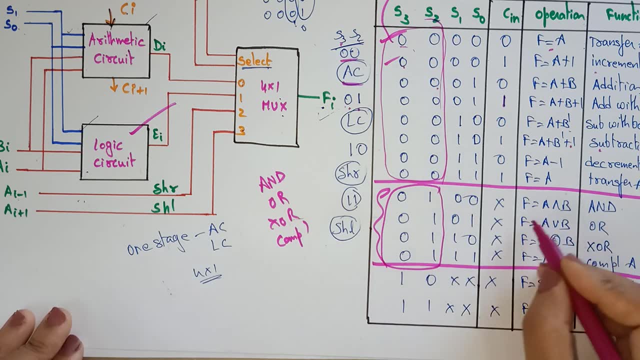 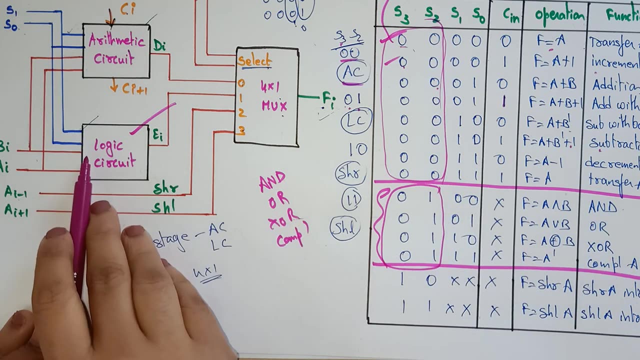 everything. it's a don't care condition. okay, so this part is a constant, because 0, s3 and s2, both are 0, 1, then only the logical operations are going to be performed. so whenever 0, 0 is there the inputs s1 and s0, if s1 and s0, the selection bits is of 0, 0, 0, 0, then it is going to perform. 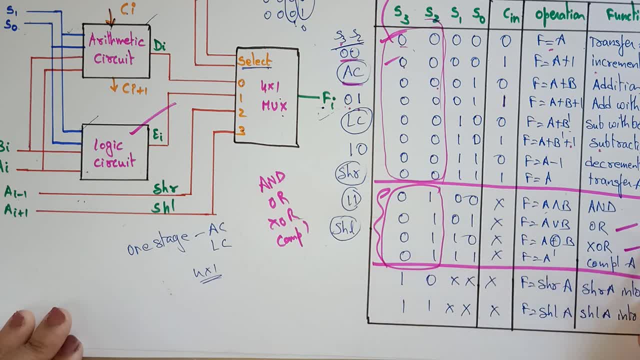 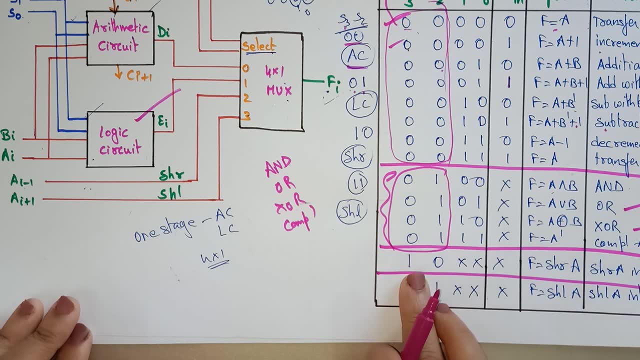 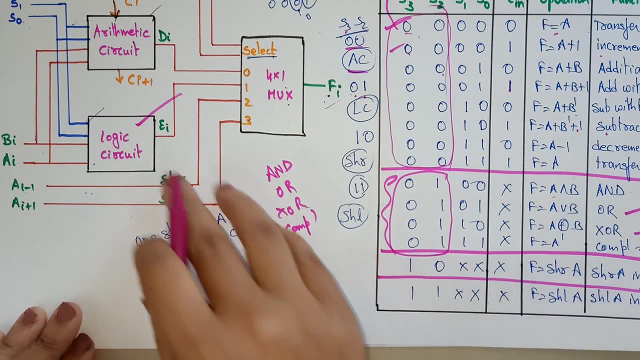 and operation 0, 1 or operation 1, 0, x or 1: 1 complement. okay, now, coming to 1: 0, if s3 and s2 or 1: 0, what operation is going to be performed? shift right. so in the shift right, we are not. 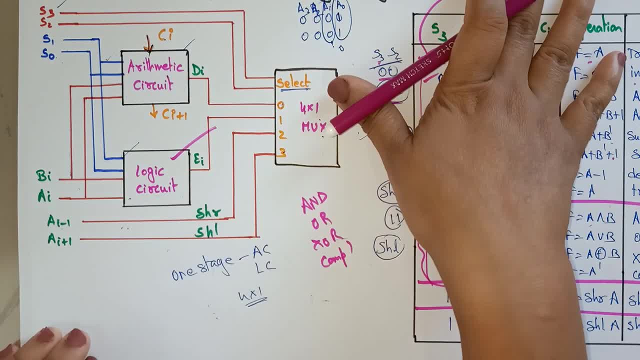 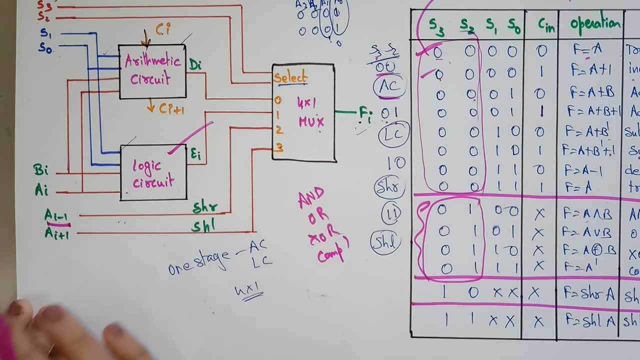 required any selection lines. s, naught and s1. we didn't require any selection lines. only it is going to shift whatever the register a is, consisting of the value that it is going to be performed and operation 0, 1 or operation 1, 0, x or 1, 1 complement. okay, now coming to. 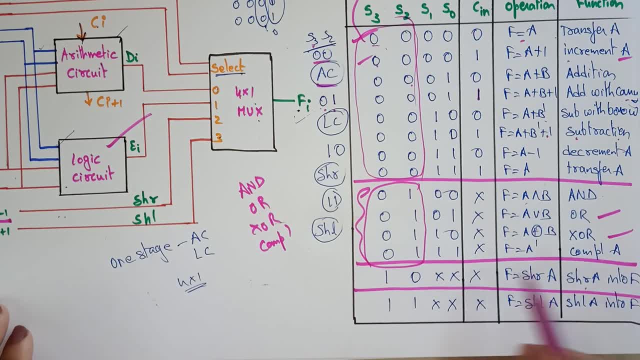 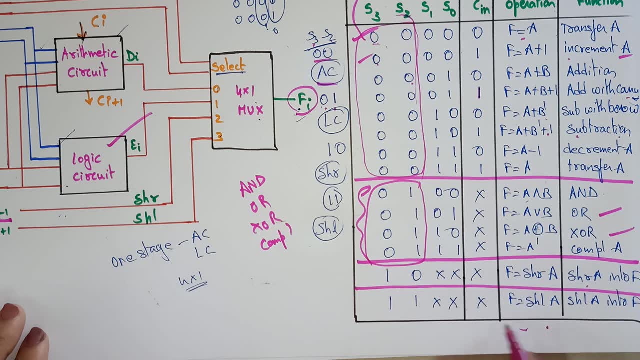 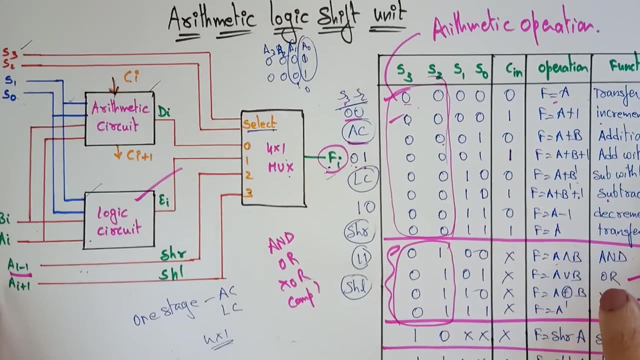 shift right, shift right a, and it will be stored in f into f. if 1, 1 is there, then it is performing the shift left and there is no carry also here, and shift left a into f. so this is what the arithmetic logic shift unit circuit. students, the one point you have to be remember that. 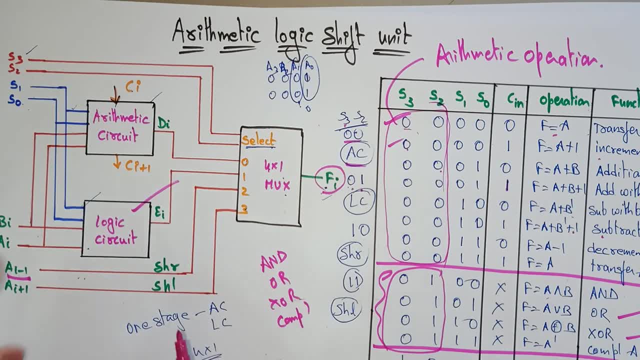 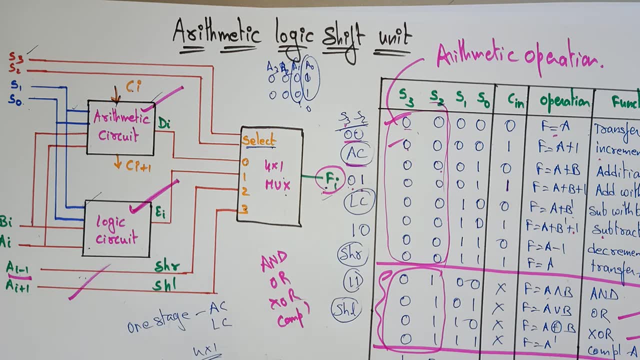 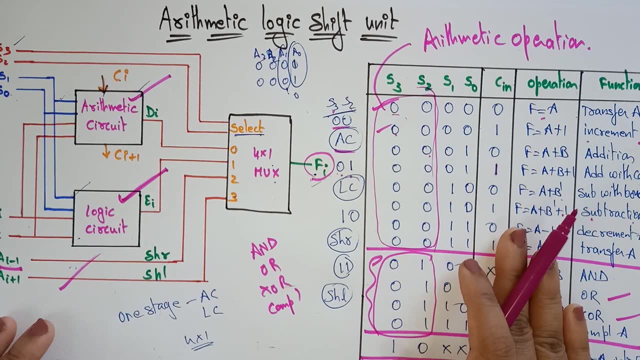 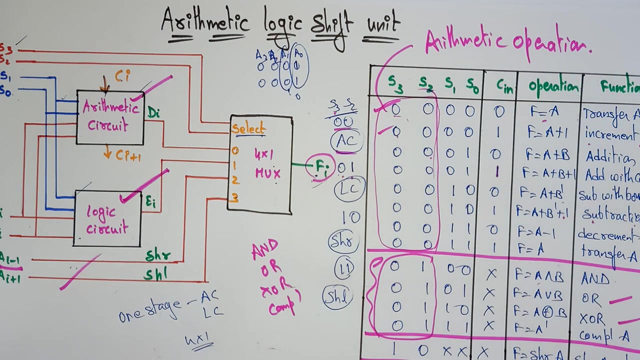 this circuit is a designed to perform arithmetic calculations, logical calculations and shift operations. so all three are performing by this circuit and these are all the inputs. based on the inputs, the operation it is going to be performed. so the carry will be considered only for the arithmetic circuit and it is not considered for the logical circuits and the shift. 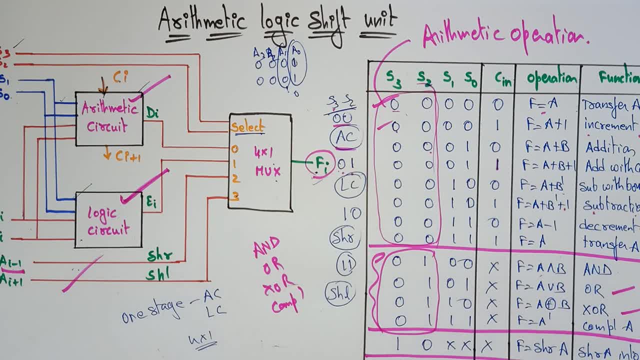 operations. so i hope you understand what exactly the arithmetic logic shift unit is. thank you.